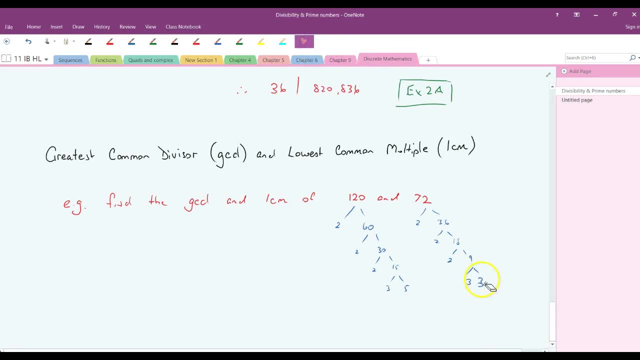 All right Now the easiest way to find your highest common factor, lowest common multiple from this position is to then draw up a Venn diagram And label each circle as one of your starting numbers. So 120 and 72. And then what we'll do is put inside here the common prime factors. So we've got 2, 2, 2. We've got three 2s that are common And we've got one 3.. Well, look at that. And what lies outside here will be a 5.. And what lies outside here will be a 3.. 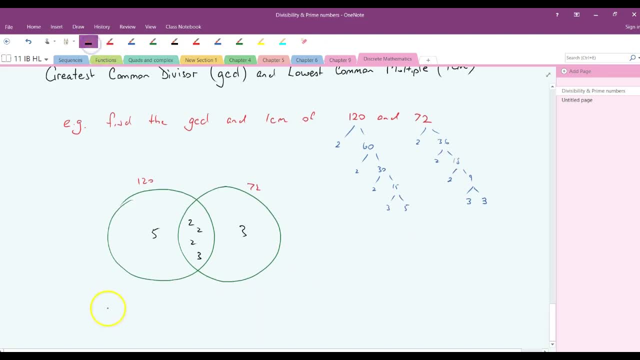 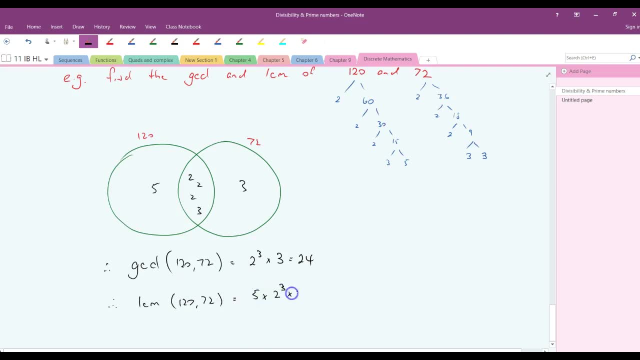 If you see, 5 by 2, cubed by 3, squared, So, that's 40 times 9,, which is 360.. 360 is the highest common multiple. So there's There's how to do that quickly, Okay. 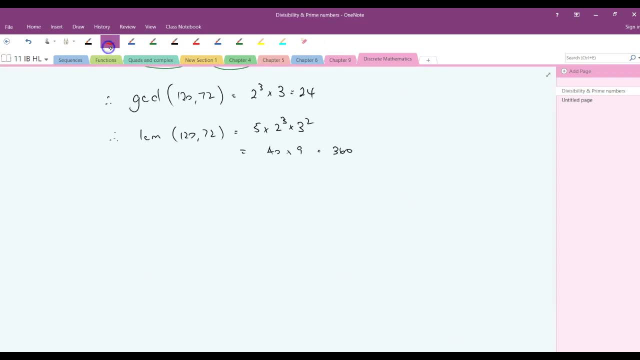 Now let's have a look at some properties here. Say, If some properties, We're talking properties, We're talking about some results, immediately, that That we can, that we can generalize. so if we say, if the GCD of two numbers, AB is equal to D, 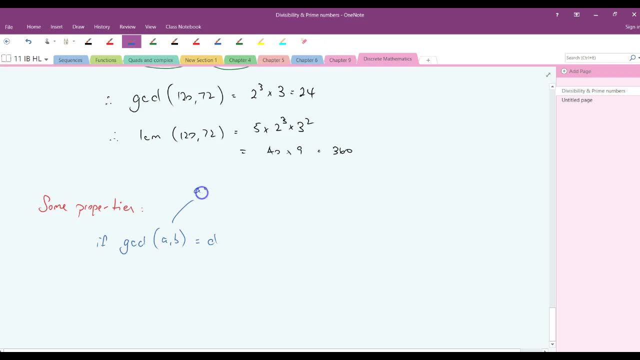 now in this case, A is going to be greater than B for these results, just to specify there- not that it really matters then. then GCD of A over D. so we divide each of these by their greatest common divisor, then the claim is that that's equal to one. now, if we ever look at our example over here- I'm, perhaps we'll look. 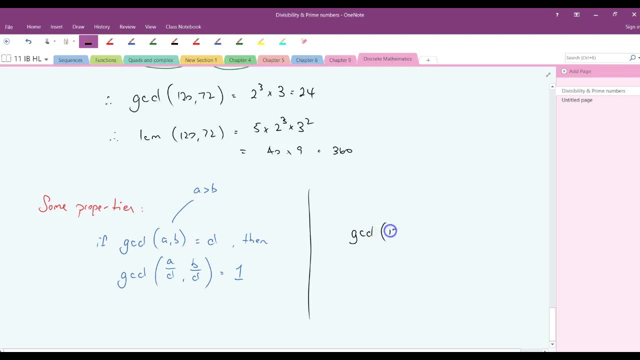 at GCD of 120 comma 75. well, we found that out to be 24, so what we do. so therefore, let's just check the GCD of 120 over 24, and it's not 75 and I, where 75 came from, 72. 72 over 24 is equal to just to. 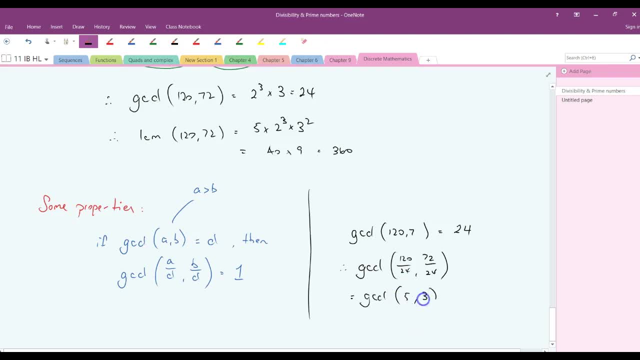 work those out, that's five three and that's equal to one. so that's that checks with that result there. if we go back let's have a look at then that's that's, that's one property. another property would be that if you the GCD on a, not if at all, the, the GCD of a and a minus B will also equal D. so 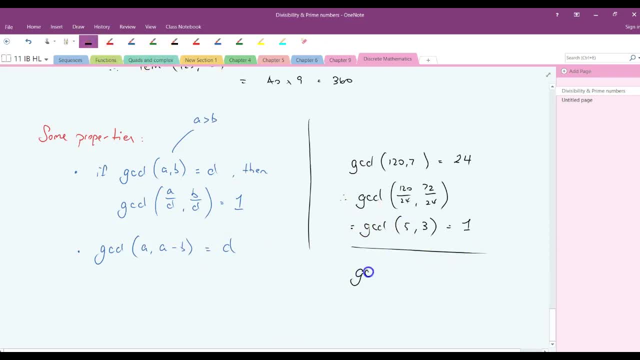 let's check that over here. that would mean over here that GCD of 120, that's 72, then a minus B, which is 48, that that would also be equal to 2, which in this case is 24, which is in fact correct. so that's fine, and 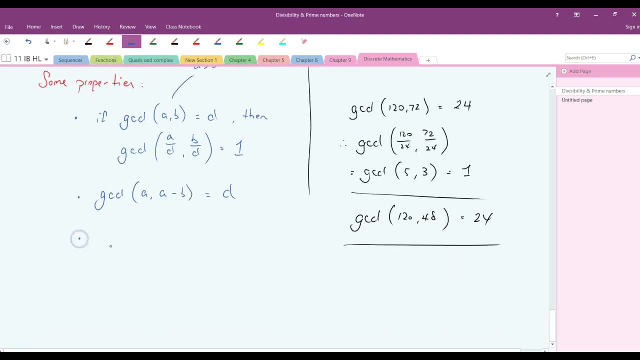 then back across. look at property number 3 here, that GCD of B and a minus QB. for some Q, some integer Q, that's also equal to D and this one's fairly fairly obvious b is guys 72. there's a minus QB, so a being 120 minus some multiple of B, so 120 minus some multiple. 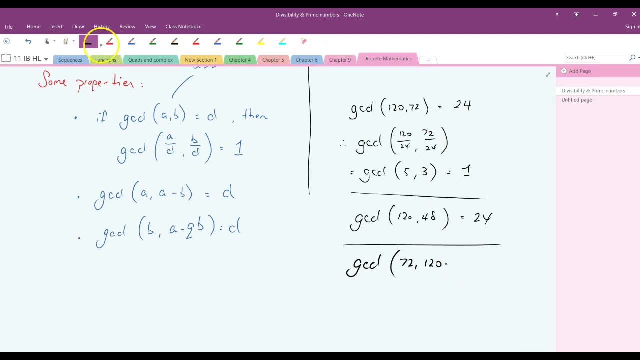 Q, some multiple of, so 48 Q. so what we get out of that is that we're always going to get before. if Q is 1, then that's 72 comma 120, that's 72 comma 120. minus 48 times 1 is 72, so that's 24, the greatest common divisor. then put 2 in. 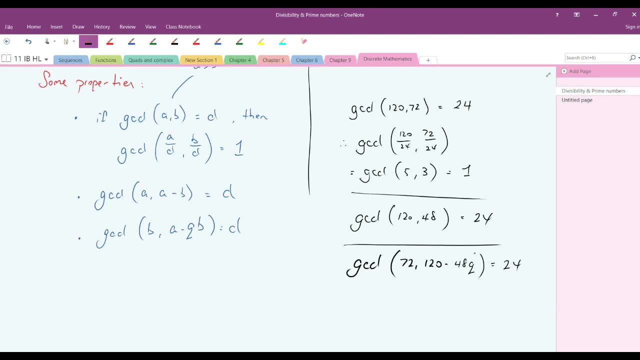 for Q, and it's 96, and then look at these GCD of 72 and 24, which is also 24, so that seems to be working out okay. so there's our, there's three properties for us to consider. okay, moving on, some more, some more properties, and this one we've, we have. 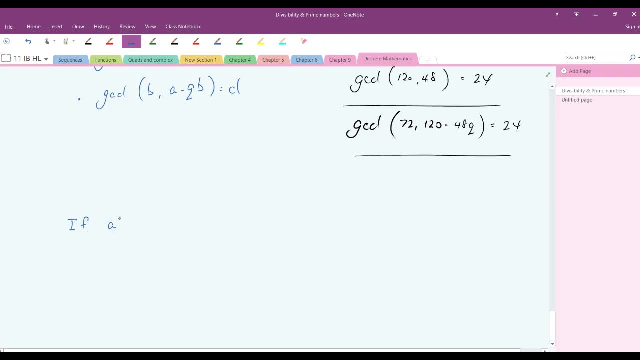 looked at if, if a is a divides n and also B divides n, I don't know, sorry than the LC M of the AB product will also divide N. If we have a look at an example of this, we have 8 divides 16, that's true, and 4 divides 16, then the LCM of 8 times 4, sorry, yeah, LCM of AB, which 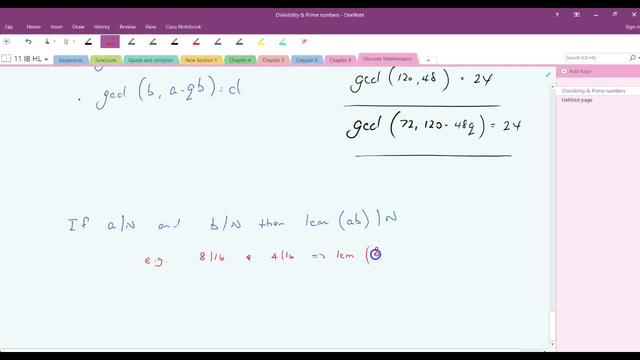 is, the LCM of 8 and 4 will also divide N. just checking that, LCM of 8 and 4 is 8, which in this case divides 16. And N is 16,- pardon me, put 16 in there, which is true. 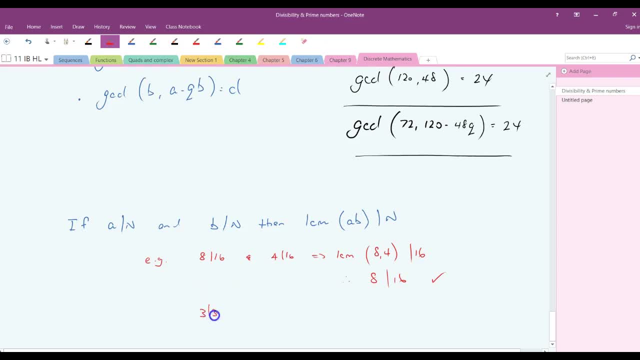 Let's have a look at, say, 3,. well, we know 3 divides 36, and we also know that 4 divides 36, so therefore, the LCM of 3 times 4, which is 12, and we know that 12 also divides 36.. 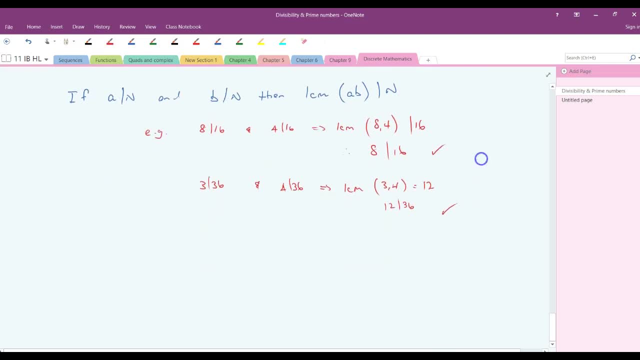 So that's, that's, that's correct, Okay, moving, moving on then with another interesting, another interesting property here: that the greatest common divisor of two numbers multiplied by the lowest common multiple of same two numbers, well, that's equal to the product of those two numbers. 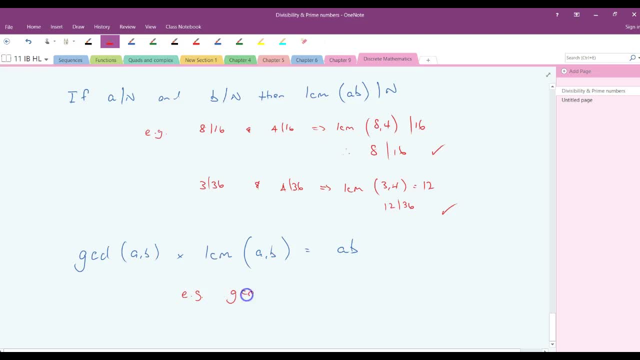 Let's see if this checks out. All right. so let's have a look at, say, the GCD of 4.. Let's have a look at the GCD of 4 and 6, and multiply by the LCM of 4 and 6,. claim is that: 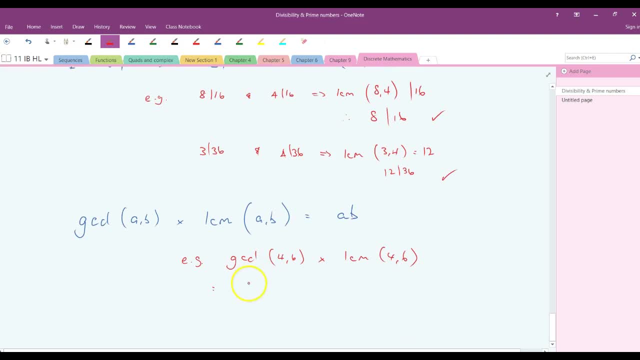 the result will be 24.. Let's look at this. the greatest common divisor? well, that's 2,, isn't it? The greatest common multiple? that's 12, 24,, which equals 4 times 6.. Seems to work. 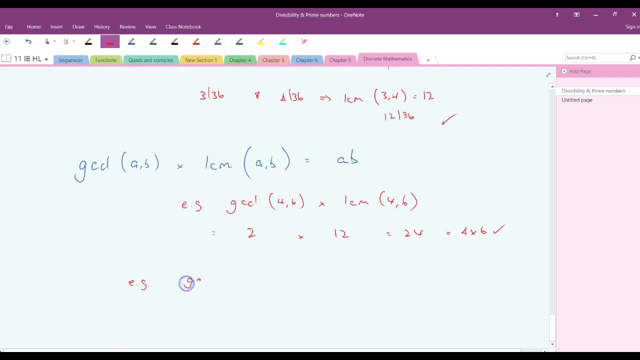 Okay, let's do another example. Let's look at the GCD of 8 and 14, and we'll multiply it by the lowest common multiple of 8 and 14.. Is that going to equal 8 times 14,, 112?? 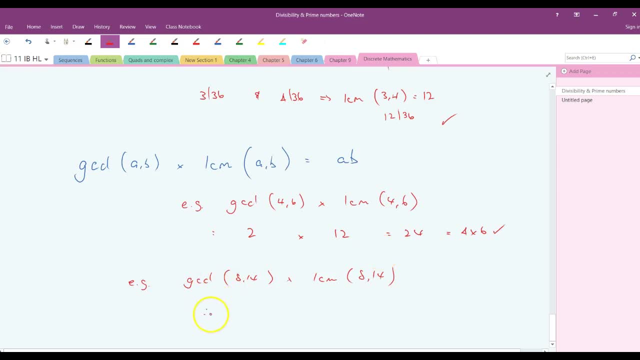 Okay, Well, the greatest common divisor- let's say it's- equals. the greatest common divisor is again 2,. 2 goes in there. the lowest common multiple of 8 and 14 is 56,, so that's 112,, which is equal to 8 times 14, so that works too. 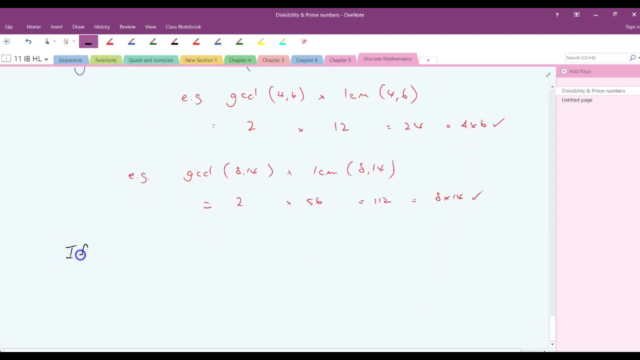 And finally, finally, if- and we've looked at this one before, actually if A and B are. we looked at this in the last section. But just to recap it, if A and B are relatively prime, looking at a couple of results here: 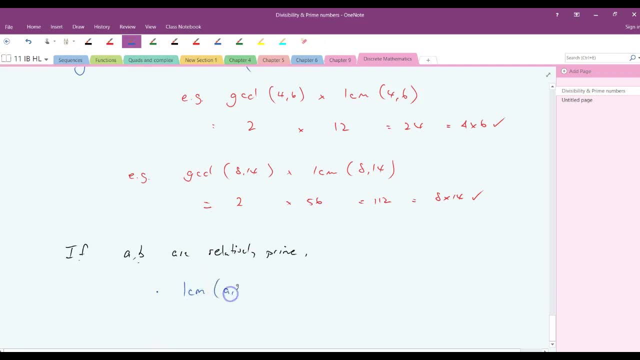 we're looking at. the LCM, therefore, of AB is equal to AB. that's a little example here- If they're relatively prime. so LCM of 2 and 14.. Okay, Of 2 and 7,, which are relatively prime, well, that's just equal to 14,, isn't it say? 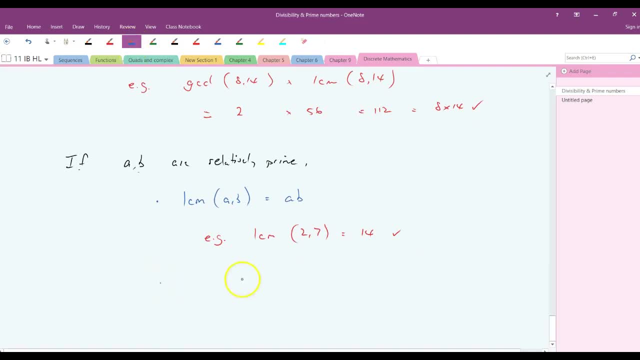 That's just 2 times 7, so that's fairly easy to believe. And then if A divides N- and this is the one that I was referring to a second ago that we looked at in the previous section on divisibility- If A divides N and B divides N, then AB, the product, will also divide N. 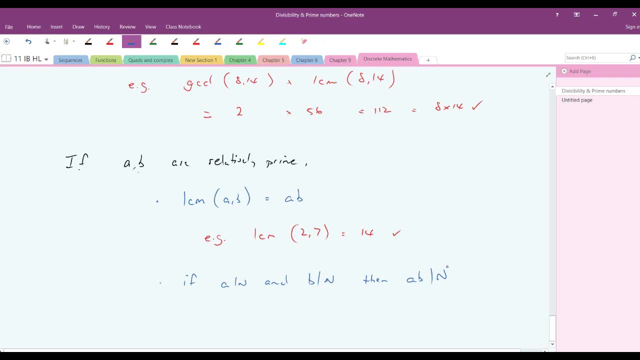 Okay, Let's launch, Let's launch. Okay, Let's launch into exercise 2B and we'll look at that in class Cheers.